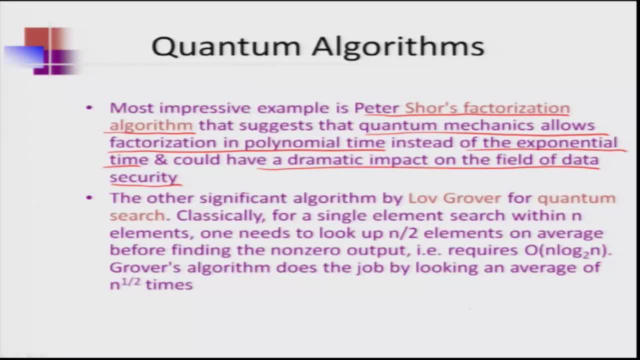 basically available, then it would mean that the data security which is basically based on the idea of prime factorization with a large number, is going to have a lot of difficulty in maintaining security. So that is why this particular problem is very interesting to look at On one side. it also provides, on the other side, better ways of creating cryptography. 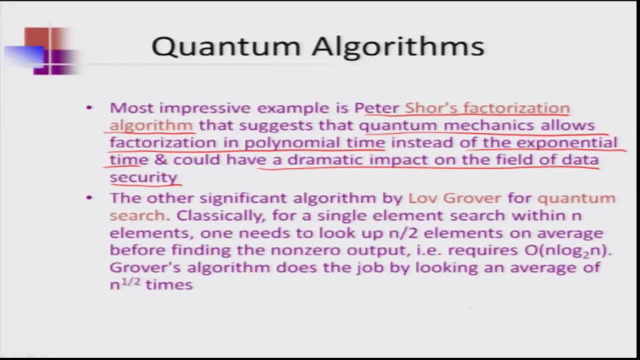 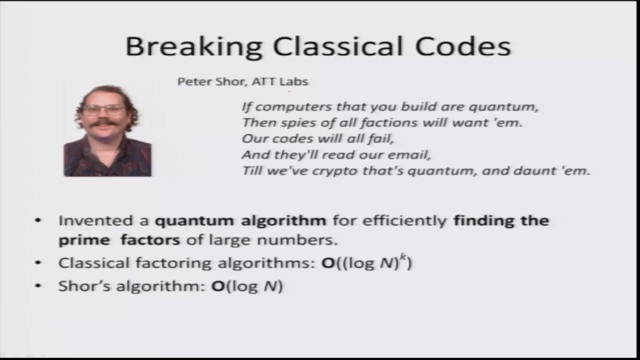 because if you can do this kind of exploration, So Pais Gattik, as he mentioned, they will be having all the benefit and our security goes. but on the other hand, once we have the quantum on our side also, then we can. 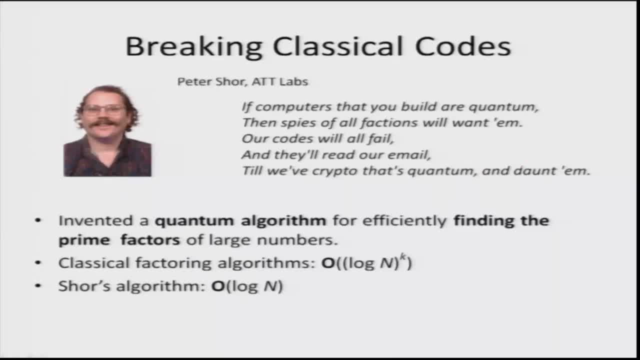 keep it so secure that, once again, nobody can read them. So that is the reason of pursuing this particular concept of security through quantum aspects. So he invented a quantum algorithm for efficiently finding the prime factorization. The classical factoring algorithms work in the order which is exponential in time, whereas 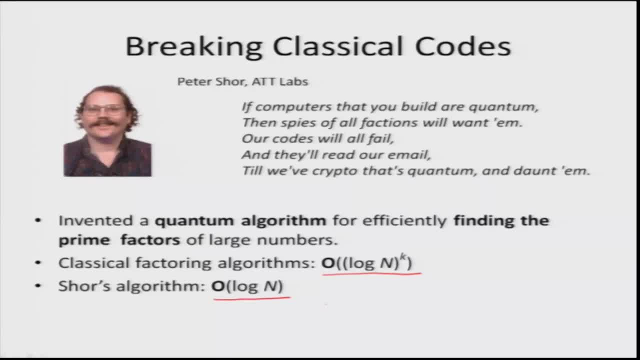 the Shor's algorithm works in polynomial time and therefore it is so impressive. and that is exactly the utilizing the full power of the quantum, because that is expected when you do a quantum algorithm, The reason being that we all know that quantum is a very important. 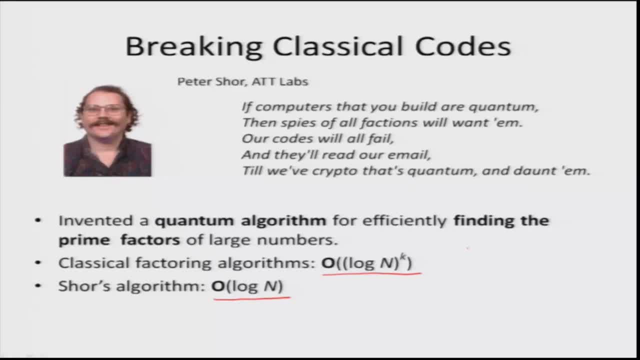 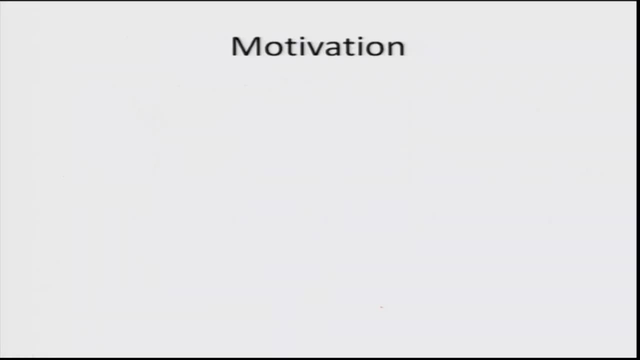 part of our life. We all know that quantum subspace is exponential in size compared to the classical subspace. That is the reason why this should have happened all the time, and here is the first case where it was actually shown. So the motivation is plenty. It is for factoring non prime integers of N of l bits and many. 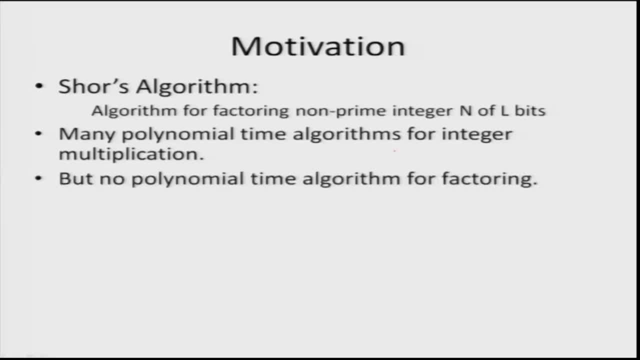 polynomial time algorithms for introducing. So these are models which we can see this for integer multiplications are available, but there are no polynomial time algorithm for factoring, because it is like, very easy to find the solution of two numbers which are being multiplied, which can be primes, but to be able to get the solution or the 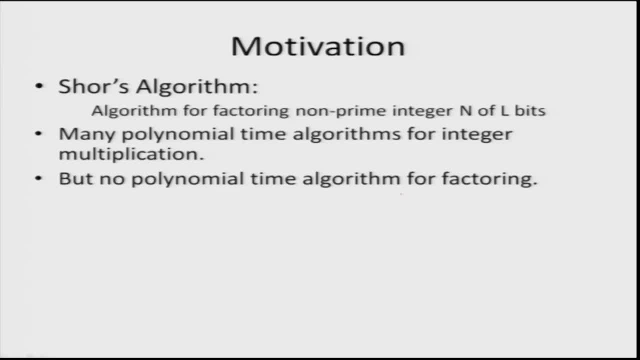 factorization of a large number into its primes is a hard problem. Quantum algorithms are faster than classical algorithms. that is what we will show. Algorithm is based on quantum Fourier transform, So this is one of the things which we will also learn as a part of this particular algorithm where we will be learning about quantum Fourier. 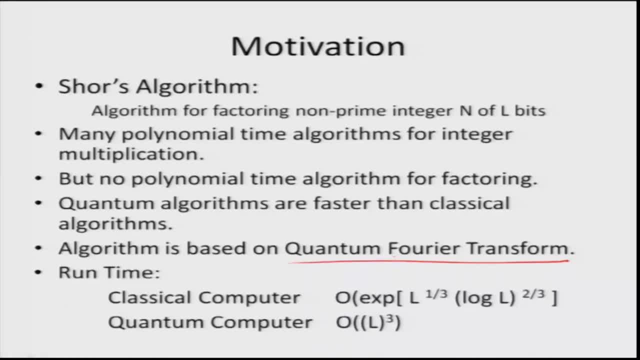 transform. The run time is the biggest advantage, as we have been discussing before. For a classical case it is exponential, whereas in the quantum case it is polynomial. So the exponential comes because I have a log sitting here and an exponential sitting. 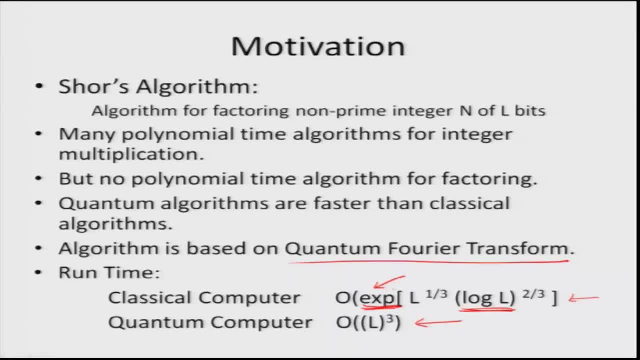 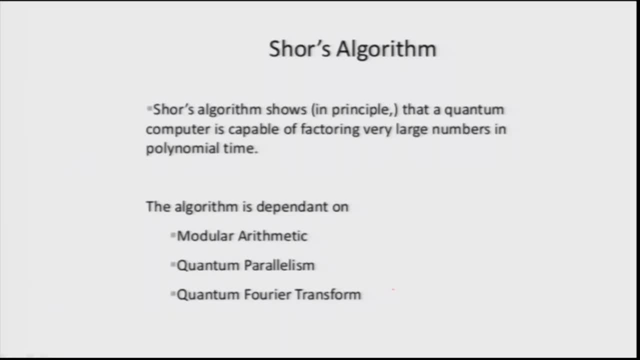 here. This is the reason for our exponential. So the source algorithm shows in principle that a quantum computer is capable of factoring very large numbers in polynomial time. The algorithm is dependent on modular arithmetic principles, quantum parallelism and quantum Fourier transform. 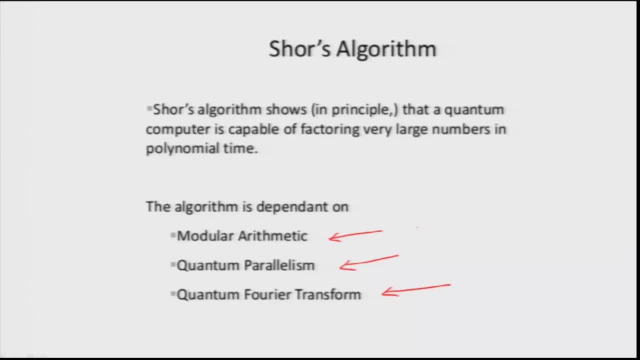 So the first part, which is modular arithmetic, is essentially classical. there is nothing new in it. The quantum parallelism is the part which is quantum and obviously the quantum Fourier transform is also the part which is quantum. So the entire algorithm therefore has essentially parts. some of it remains classical, as expected, So the problem can. 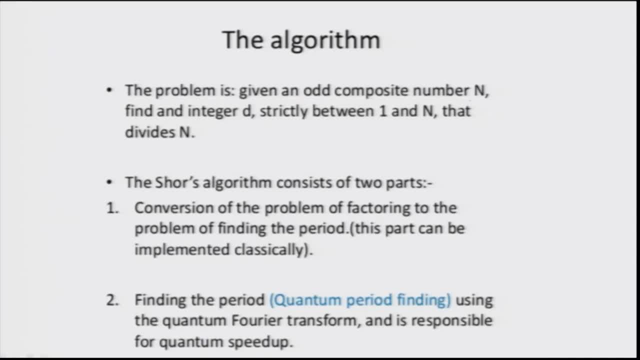 be stated in such a way: given an odd composite number, n, find an integer d strictly between 1 and n that divides n. The source algorithm consists of mainly two parts: conversion of the problem of factoring to the problem of finding the period. This part can be implemented. 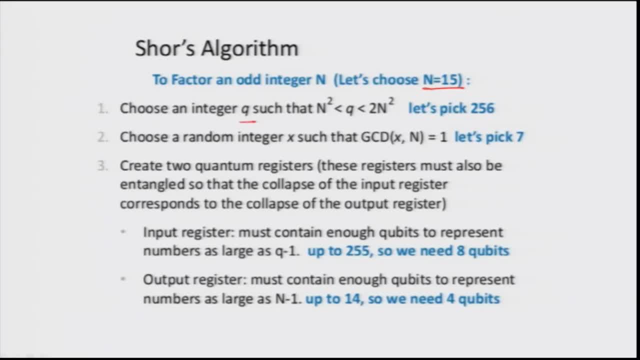 have to choose an integer, q, such that now, q, such that it lies in between n squared and 2, n squared. that is what we said. So it can be any number. let us pick up 256, because it is 256 power, something You choose, a random number, x, such that the GCD of x, n is 1.. So we 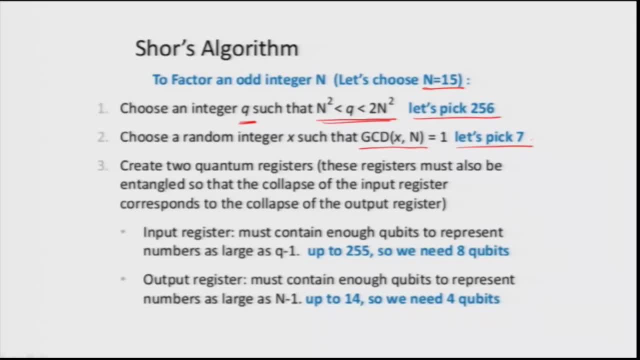 can pick a number like 7, which we did earlier Create two quantum registers. these registers must also be entangled Now. we have discussed about entanglement before, and that is the part which is critical in Schorr's algorithm. We will again revisit that in slightly more. 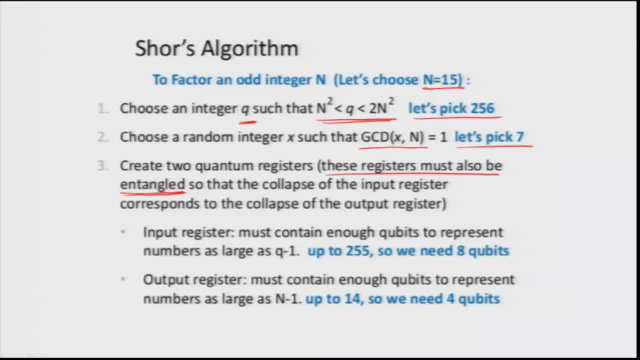 detail later on one, but for now just look up your notes or previous lectures to go back to understanding what entanglement is. So these registers have to be entangled so that the collapse of the input register corresponds to the collapse of the output register, right? I mean this. 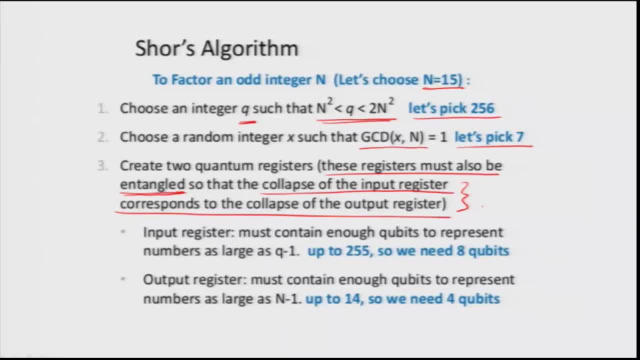 is the criticality of entanglement, that one process essentially ensures that the other one is also correlated one way or the other. The input register, therefore, must contain enough qubits to represent numbers as large as q to the q minus 1, that is up to 255 in this particular case. So we need 8 qubits. 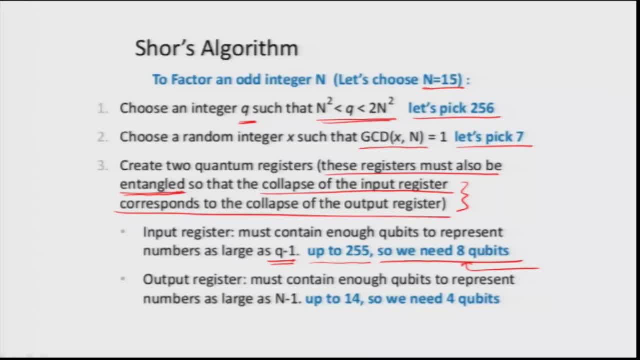 2 to the power 3 qubits which would, which can give us up to 255.. So we need we need the input register to contain enough qubits. So each she needed 2 to the power 3 to the power 4 qubits to represent numbers as large. 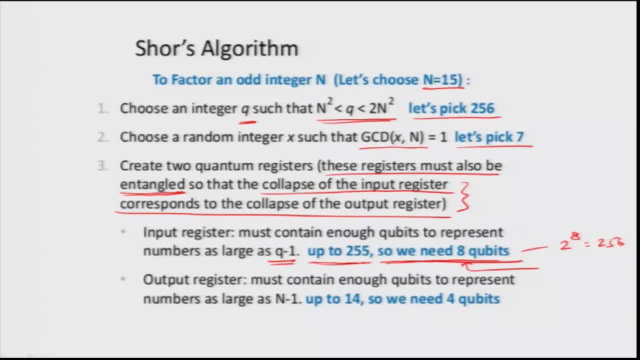 as q to the power as large as q minus 1, which is up to 255.. So that we need 8 qubits, since to the power, 8 is 256. And therefore we choose the number of qubits as 8.. 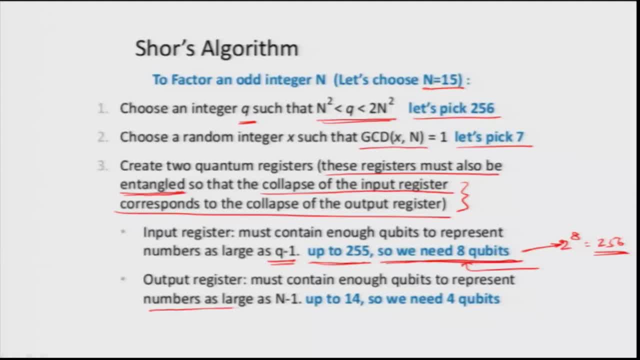 The output register again must contain enough qubits to represent numbers as large is as minus 1 up to 14.. So we basically need 4 qubits is to the power. 4 is good enough to issue. So this qubits represents a certain number guys as big as 15, and thus the number. 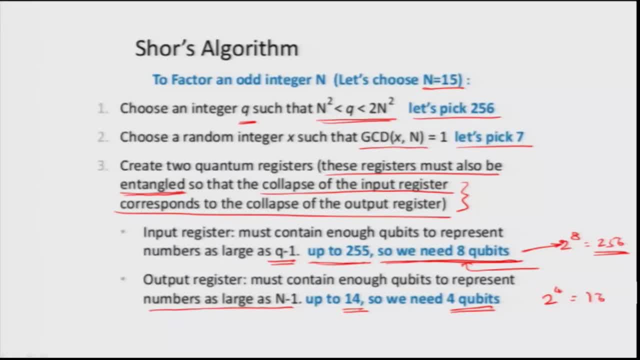 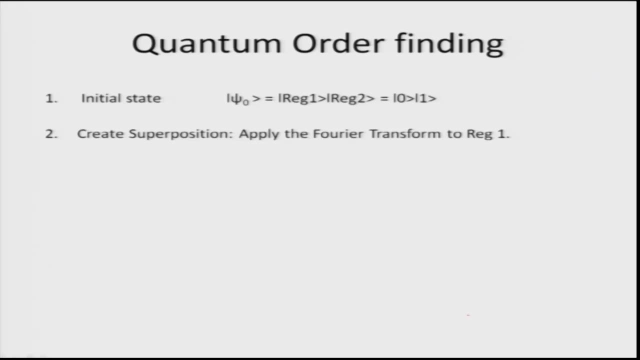 go up to 128, that is more than what we need Now in order to look at the problem of order finding, quantum order finding. let us now go back and look at how the states can be set up. So let us set up the states 0 and 1 in register 1 and register 2, which is our. 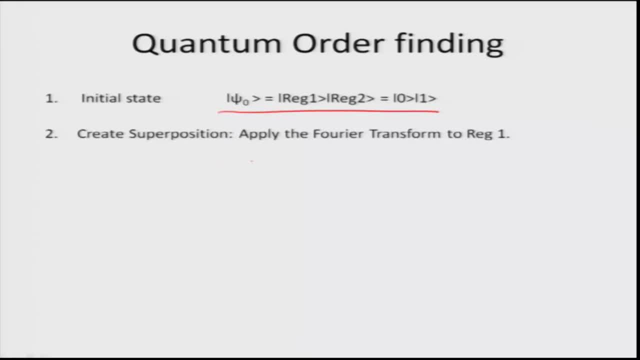 initial state, We create a superposition, that is, we apply Fourier transform to register 1.. Now, this principle of Fourier transform is something which is perhaps known to you from previous studies, but if not, we have a separate lecture where we will be focusing on Fourier transform and the quantum Fourier transform. 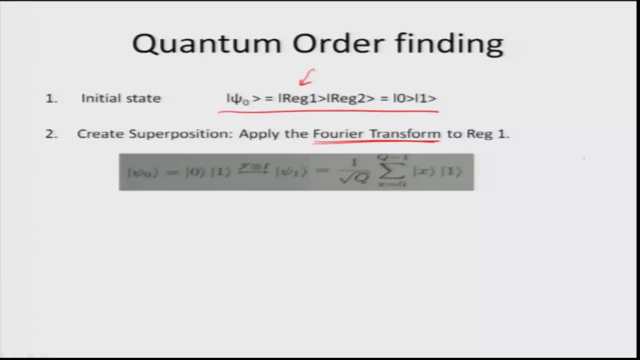 principles. However, it comes under the basics of the mathematical formulations that we have been mentioning before, So we can look back on to that once again if necessary. So once you apply the Fourier transform argument, then what you will have is: you will have: 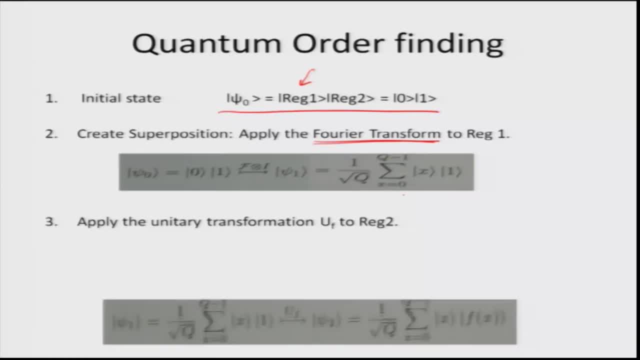 this entire state, This entire state which would look like this: And then we can apply the unitary transformation to the register 2, which is u of f, to register 2, which takes it to this functional f starting instead of the 1 function. So this is our unitary function, which puts in the f of x. 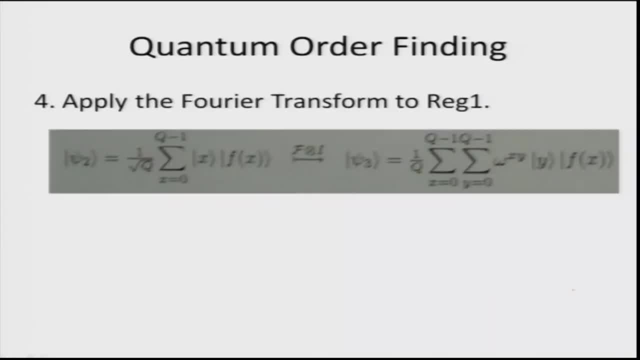 there. So once we get this form, then we can actually apply the Fourier transform again to register 1, which is x, and we are going to get this as our Fourier transform argument. as a result of application of the Fourier transform, We make a measurement on the first register now. 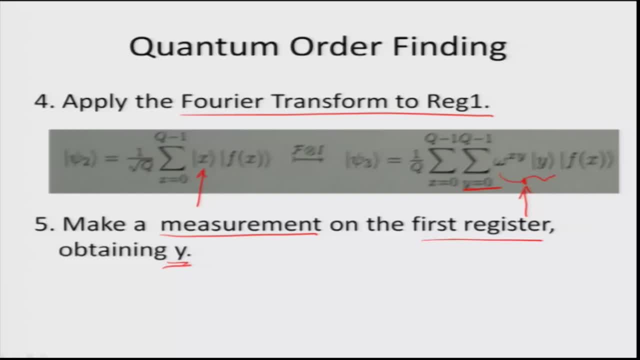 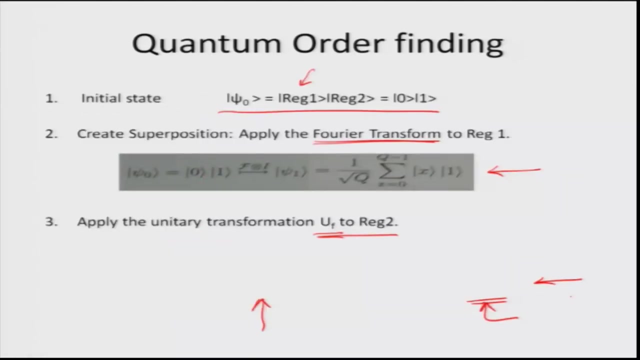 which gives us the value of 1.. y, because that is the part which we have now gotten into. We find the period P by using the continued fraction method for y over 2 to the power L. So these are the six steps which we have just discussed for your quantum part of the algorithm. So let me actually 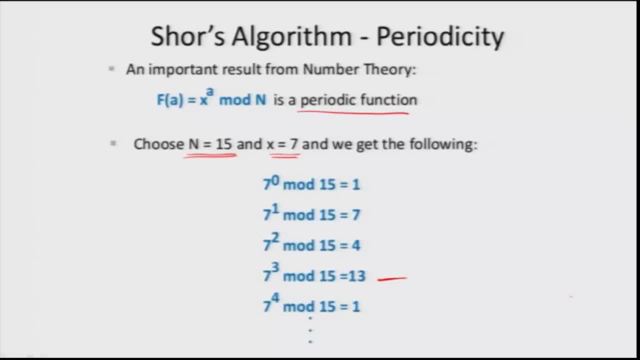 reiterate once before we close this lecture. So what did we do? We basically said that we take up a trivial case where we apply from the number theory principle, the periodic function principle, and we found out there it was possible to find out value of seven. 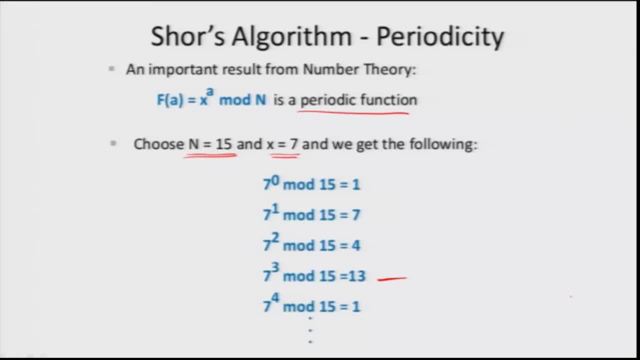 which is co-prime with fifteen, which is the number. we are trying to find out the factors for And for this particular kind of a case, where we can do each and every number in terms of finding x to the power, a mod n. we can find the periodicity by hand, because this is easy. 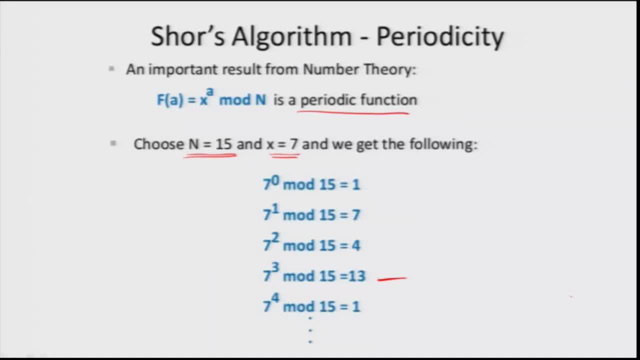 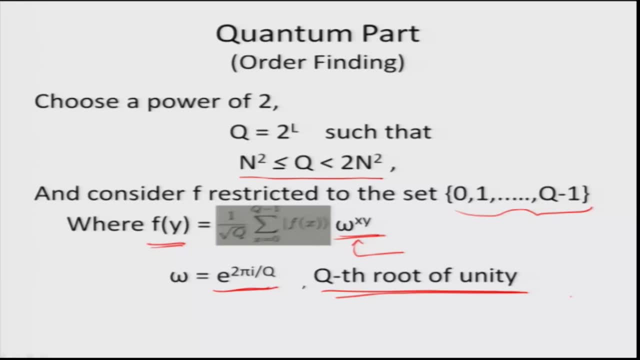 But this gives you the idea as to how we will be setting this problem up in the quantum form. So, in the quantum form, what we did was we chose the numbers and the registers in such a way so that we can set up the order finding problem. 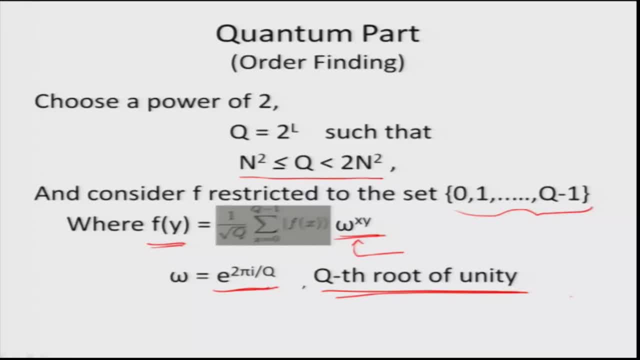 We chose in terms of powers of 2, because that is how the quantum is supposed to be. We set these functions in the sets which had the registers in those connections and we applied our functions such that we got the period function coming out, And that was possible. 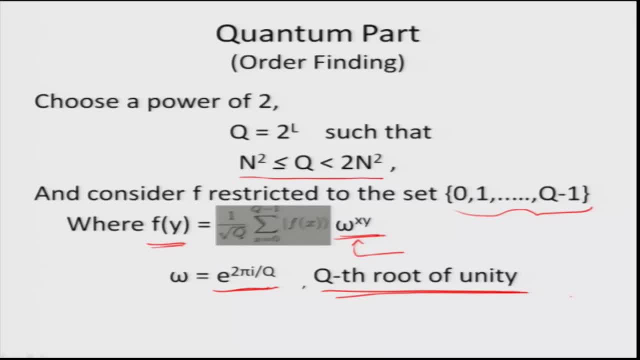 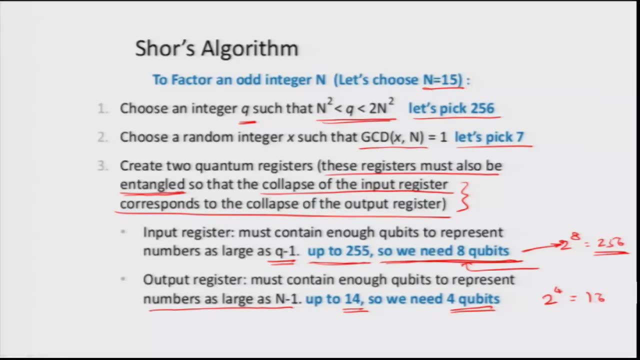 because of the application of Fourier arguments, where the phase of the problem comes into the picture. and we got the qth root of unity, for instance with the omega value here, And we went through the individual steps, in particular when we did this particular example of n equal to 15, the quantum way. So once again, even in